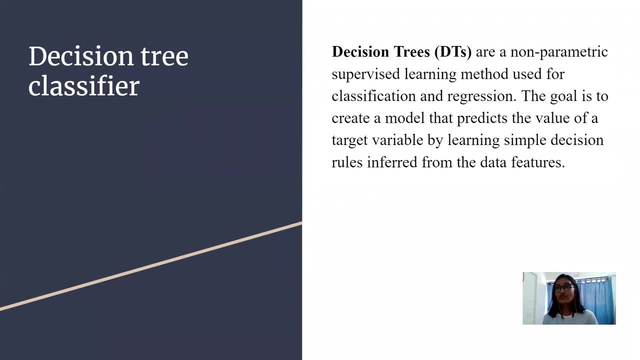 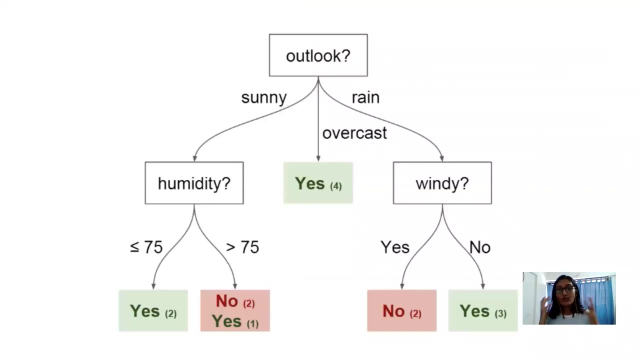 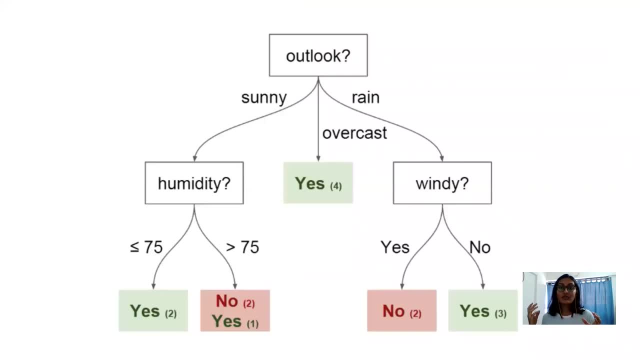 you like to go out for a walk? Would you like to go out for a walk? Would you like to go out for a walk On sunny, rain, overcast? what are the possibilities of the chances of you going out for a walk? Let's say that if you go out on a sunny day and it is humid, what are the chances that you go on? 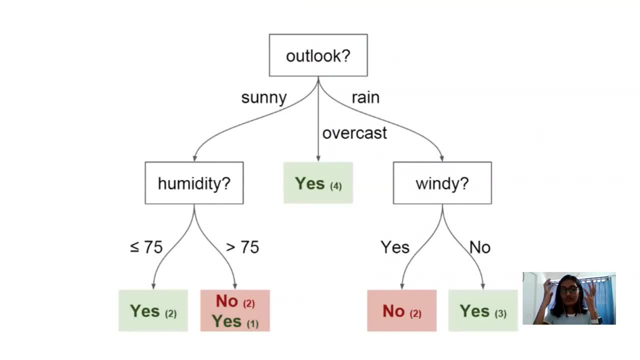 the humid day and you won't go on a humid day. So the pattern of our thinking can be jotted down as a decision tree. The logic behind the decision tree can be easily understood because it shows a flowchart type of architecture, like a tree type of architecture, which makes it 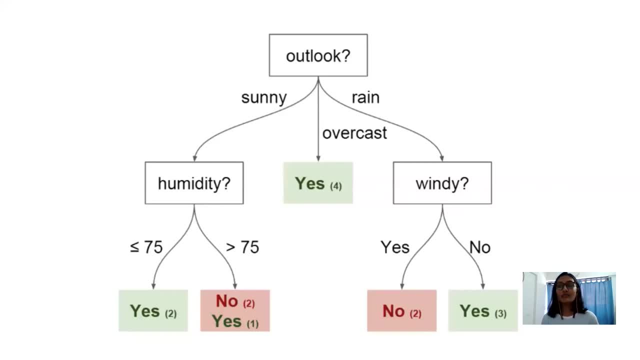 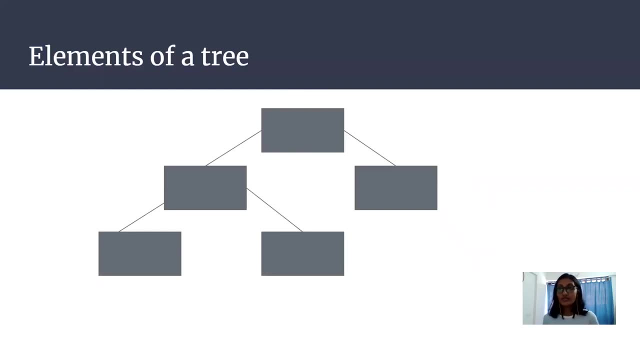 easy to visualize and extract information out of the background process. Now let us discuss the elements of a decision tree. So the different elements are nodes. So all these rectangles that you are seeing are nodes. This is the point where tree splits according to the value of. 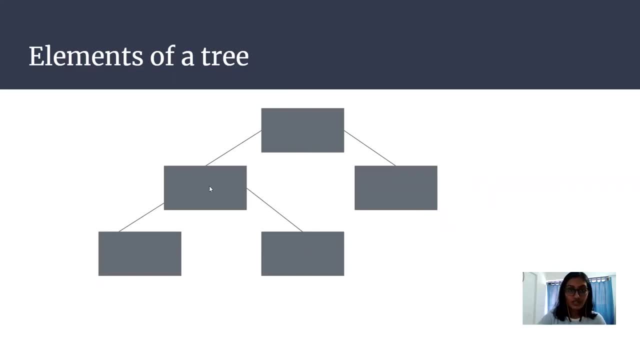 some attribute feature of the data. So these two points that you are seeing is known as simple nodes. Then we have edges. So edges, it directs the outcome of a split to the next node. we can see in the figure like this one: So from this node we are going to this node. So these all 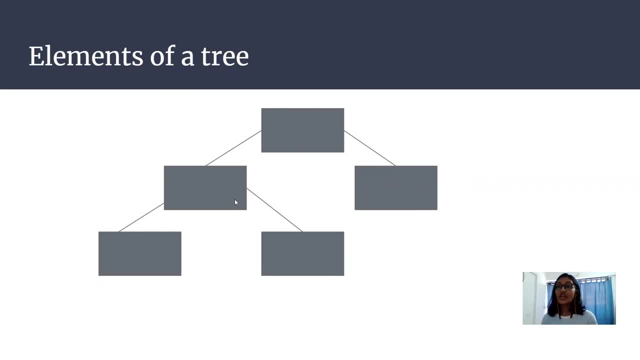 lines that you are seeing are the edges. Then we have the root. This is the node where the first split takes place. So always the head of the tree will be the root node And thereafter we have the leaves. These are the terminal nodes that predict the outcome. 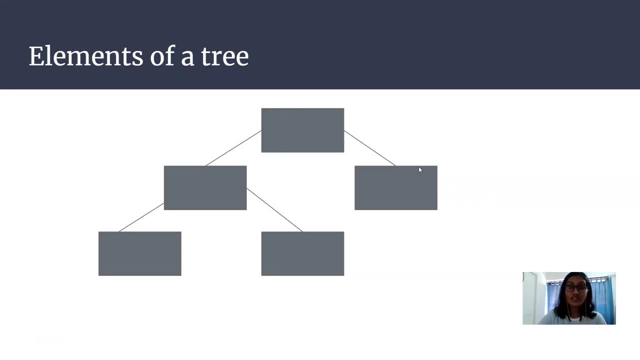 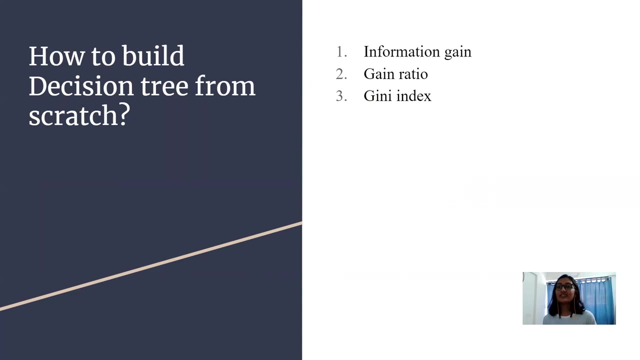 of the decision tree. So, as you can see, these two last nodes and this node here is the leaf node And, as we had discussed, leaf nodes are nothing but the data points itself. So the question arises That how should we build a decision tree from scratch? So, while building a decision, 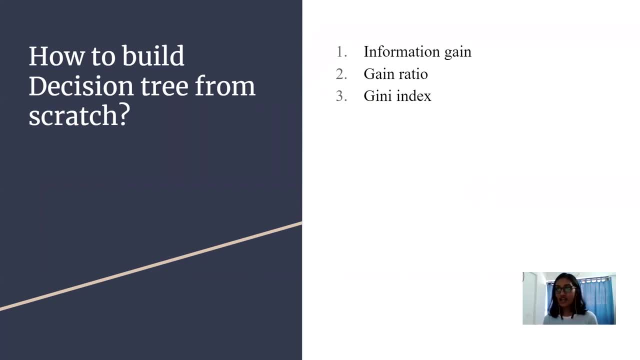 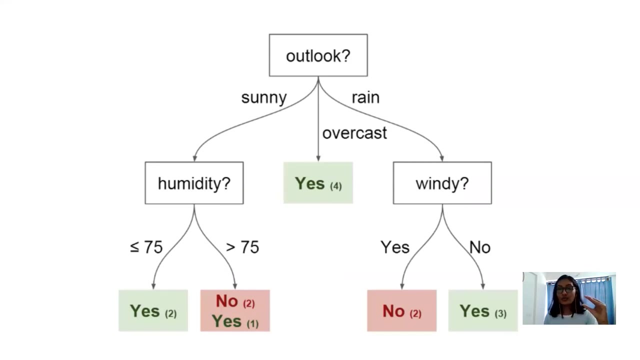 tree. the main thing is to select the best attribute from the total features list of the data set for the root node as well as the sub nodes. So, for example, if I have this diagram over here, how did I select that my humidity should be an attribute over here? 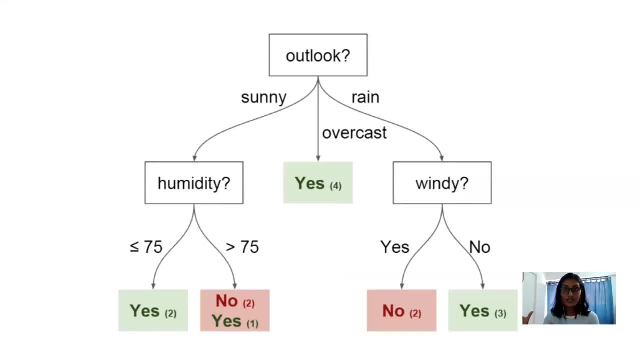 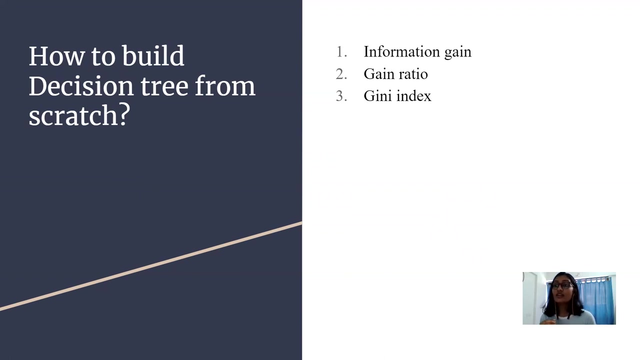 through which the splitting should be done, Or windy should be the attribute wherein the splitting should be done, Or why is not humidity the root node? So all of these questions pops up, And the answer to this is that the selection of best attribute is achieved with the help of a technique known as attribute selection measure. So with 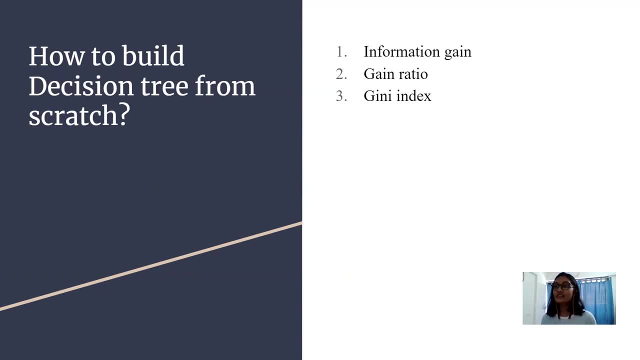 the help of attribute selection measure, we can easily select the best features for the respective nodes of the decision tree. Now the different techniques for attribute selection measures have been noted down here. First is the information gain, then we have gain ratio and thereafter we have gain index. 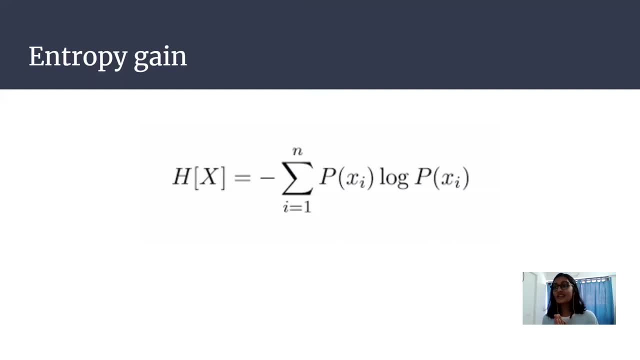 Before moving forward one should understand the meaning of term entropy. Entropy is used a lot while computing the attribute selection methods. So entropy is a measure of impurity or uncertainty. Entropy is a measure of impurity or randomness of the data. So we will get a better idea. 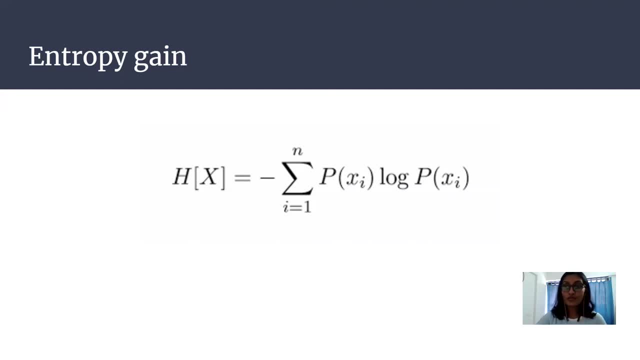 of entropy in a further discussion. But entropy, the formula for entropy, has been given over here, So xi. here are the number of classes that we have, like, yes or no, windy, humid, sunny, all of these can be the classes And we are finding the probability of that class multiplied. 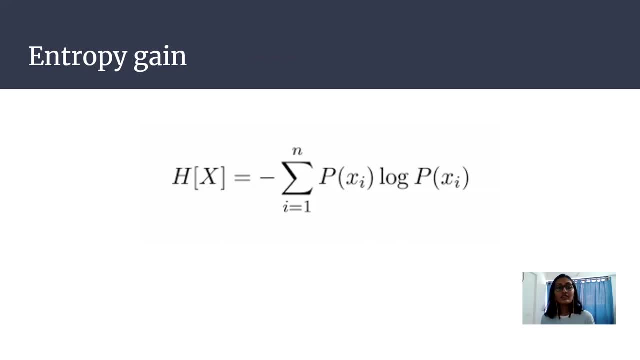 by log to the base of probability of that class. So this is what our entropy is. Let us now understand the very first ASM technique, which is information gain, which is also known as ID3 decision tree. So information gain is the measurement of changes in entropy value. 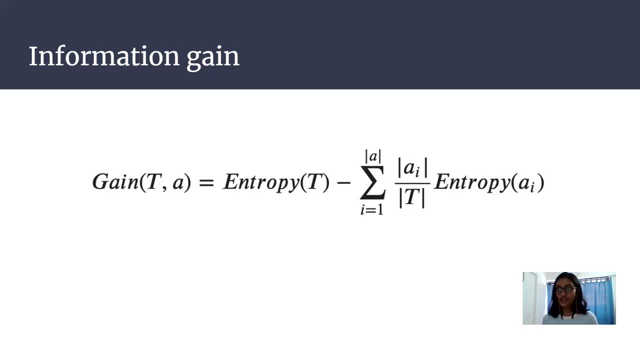 after the splitting or segmentation of the data based on the attribute. So it tells us how much information or attribute providers following the value of information gain, splitting of the node and decision tree building is being done. so decision tree always tries to maximize the value of information gain and a node attribute having the highest value of information gain. 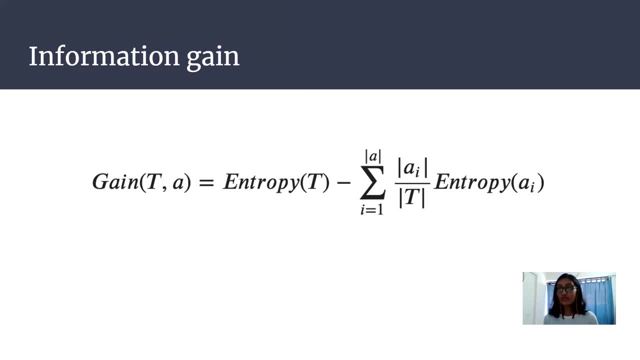 is being split first, so information gain can be calculated as the formula which is being given over here: entropy, as we have calculated in this formula, and this is the weighted average. so these are the data points and this will be the summation of all the data points. so 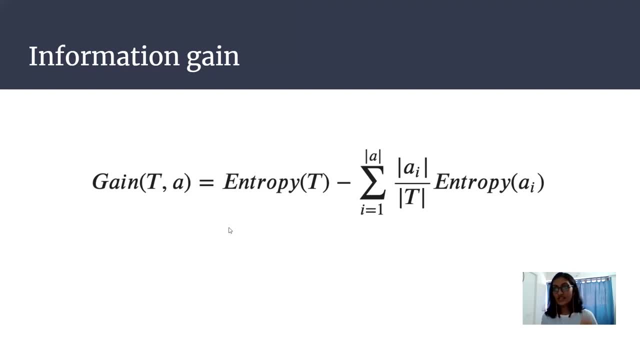 this is the gain that we are finding thus revising the procedure. we will first compute the information provided by required to classify tuples of t, like yes or no. thereafter, you will be computing information gain for each attribute, like windy humidity, humidity and humidity, etc. thereafter, you will be computing the formula, this one, the formula which is: 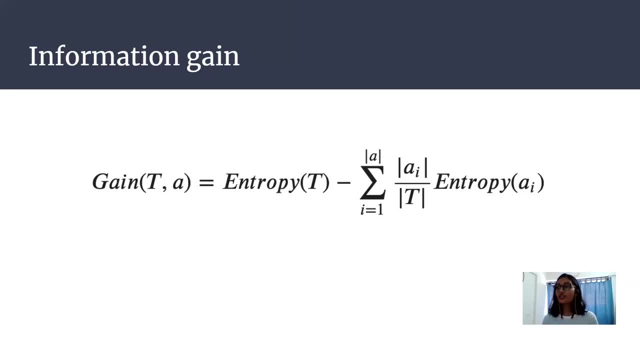 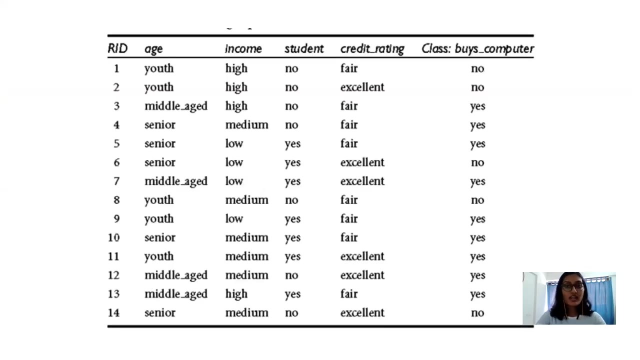 given over here. then attribute is chosen on the basis of information gain. higher the information gain, greater is the possibility for it to be selected as a node. now let us take an example. imagine that this is the data that has been given to us now in the different columns we 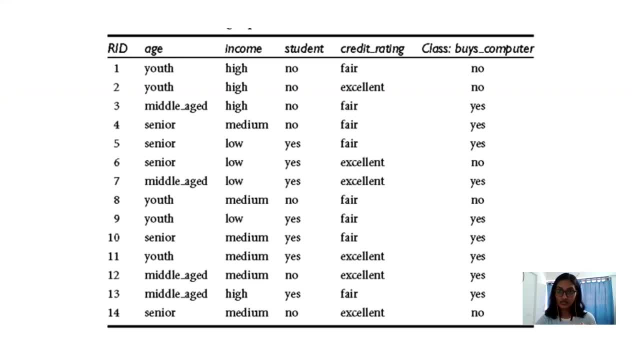 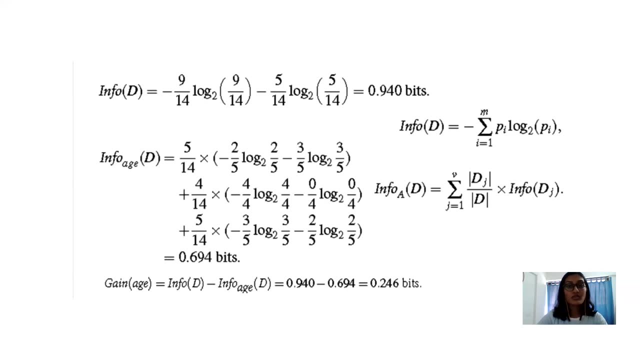 have is age, income, student, credit rating and all these columns are the reasons through which we are getting the two pluses, whether yes or no, whether the person will buy the computer or not. so what do we do? is we first of all find the information gain of yes and 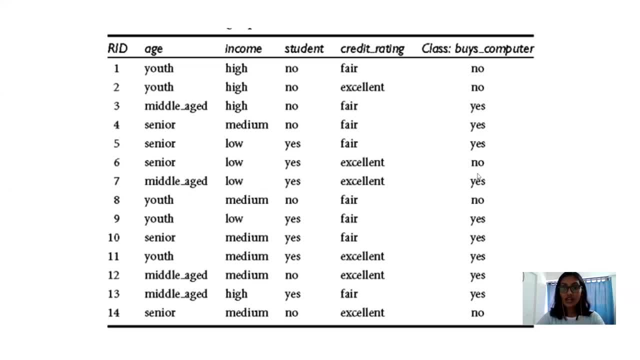 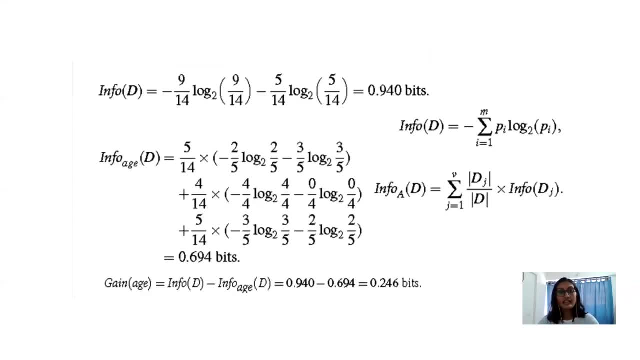 no. so here, if you observe, these are, these are the attributes that we have. we have 14 values, 9 of them is yes, and then we have 14 values and 9 of them is yes. so that means rest are no, and that is how the very first thing is being calculated. thus we 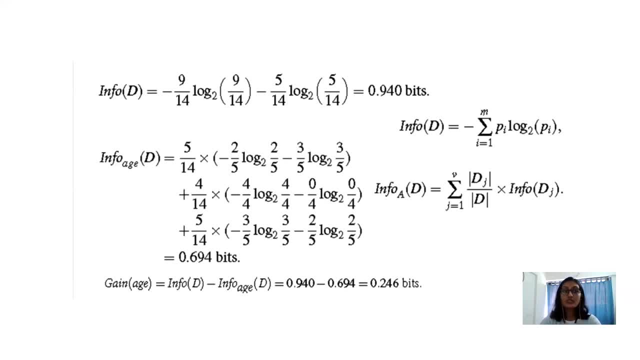 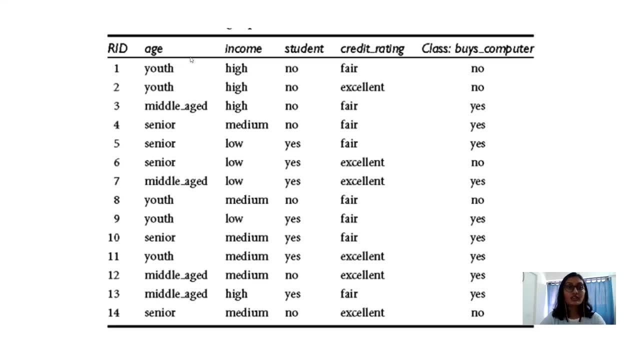 have found out the entropy of the classes. thereafter we will be finding entropy for each of these columns. so first of all we are finding the entropy for the column age. so for the age, this is how we are calculating. where in this is the weighted average of? here we have three different types: youth, middle-aged. 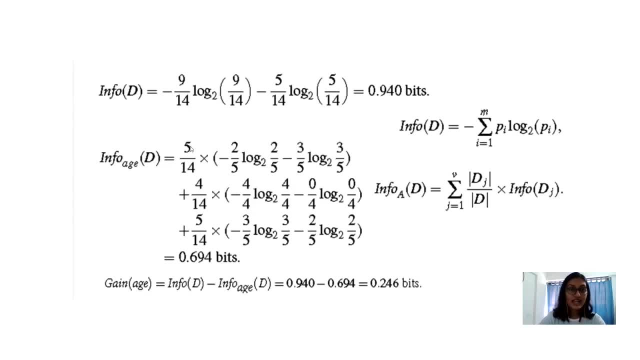 seniors, right? so we are just adding the number five for youth and how many out of the youth are yes and no? that is the entropy that we are calculating. thereafter we are going from middle-aged and thereafter we are going for senior. after getting this, we are finding the gain of age. so we are subtracting the. 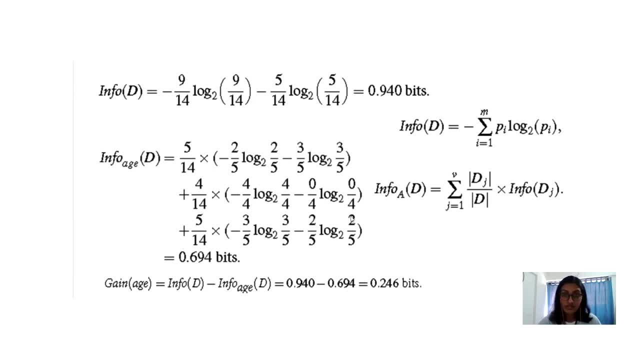 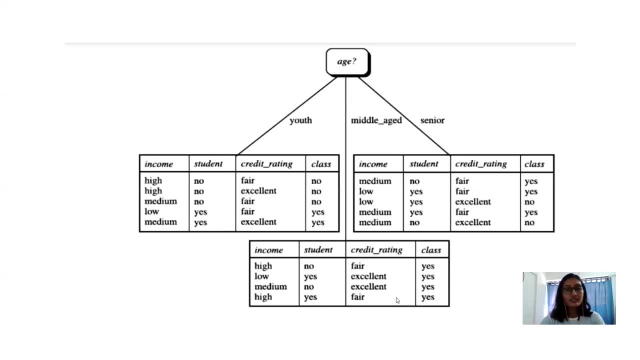 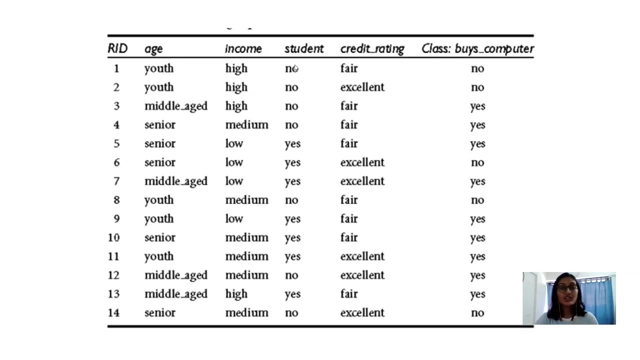 value that we got over here, which is point six, nine four bit from this value and the answer that we are getting as point two, four, six bits. so this is the kind of table that we have got. in actual sense, you have to find the gain for age, income, students, credit rating, everything, and 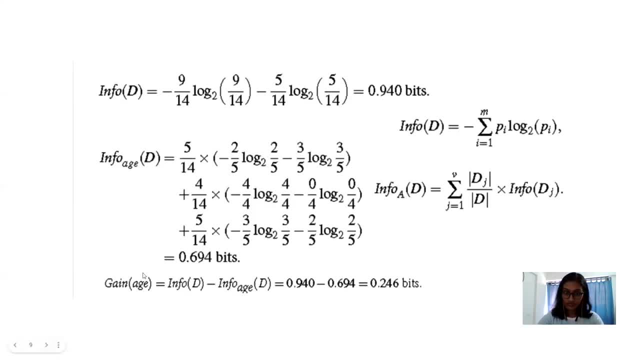 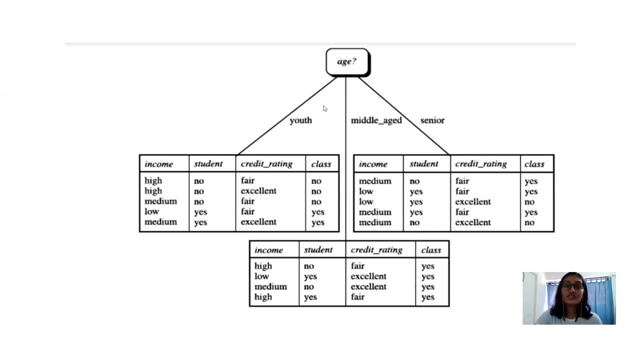 thereafter you have to prepare the gains that you are getting. but since I have already done that, we find out that gain of age is great over here, and that is how we are getting history as the output and after dividing and splitting age into Hooth, middle-aged, non-meaning and middle-aged, non-meaning and middle-aged. 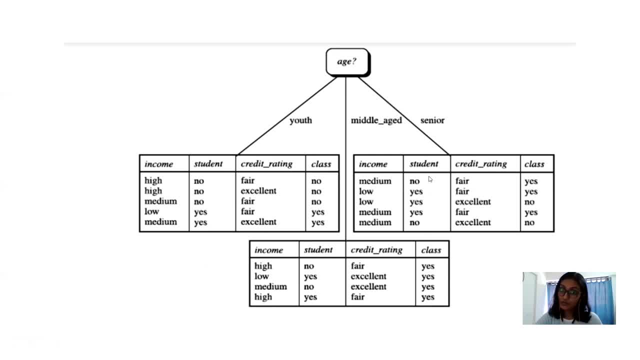 and senior. we have these as our tables. now, for each of the table that you are seeing over here, we have to again do the whole process of finding the gate, and that is how the whole tree is being made. so i hope this is clear to you now, one of the only limitation that this method, which is 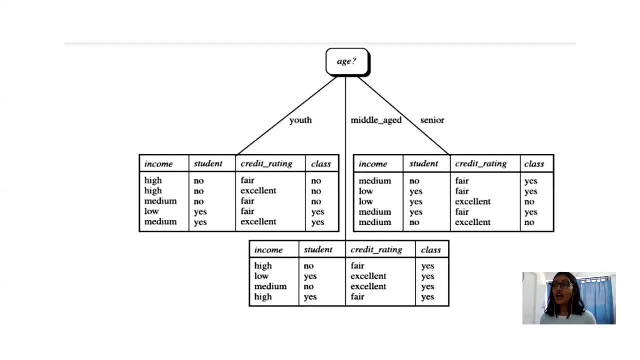 id3 decision tree has is that it is biased towards multi-weighted attribute. the information gain measure is biased towards tests with many outcomes. that is, it prefers to select attributes having a large number of values. for example, consider the attribute that acts as a unique identifier, such as a product id, a split on product id. 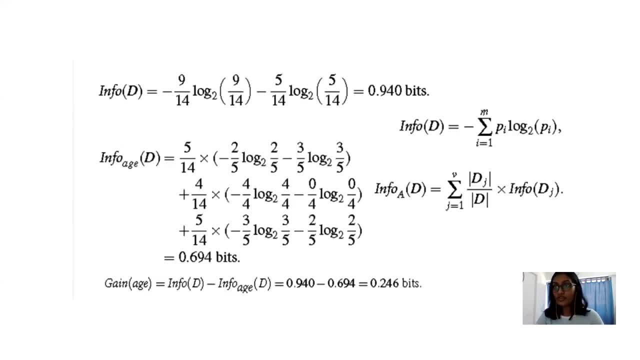 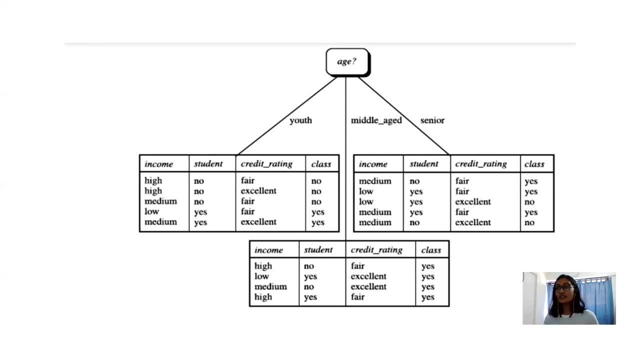 which we have over here, the leftmost column. so a split of product id would result in large number of partitions and each one containing just one table. because each partition is pure, the information required to classify said d based on the partitioning, would be: information: grain of product. 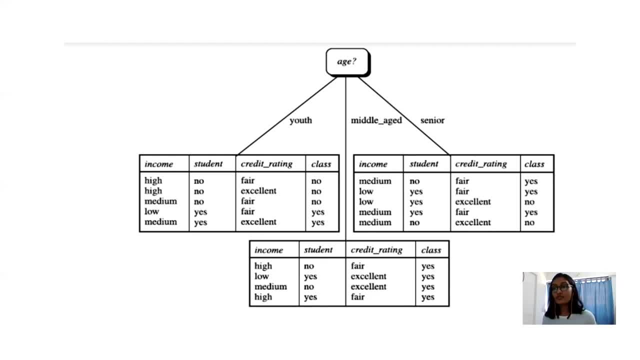 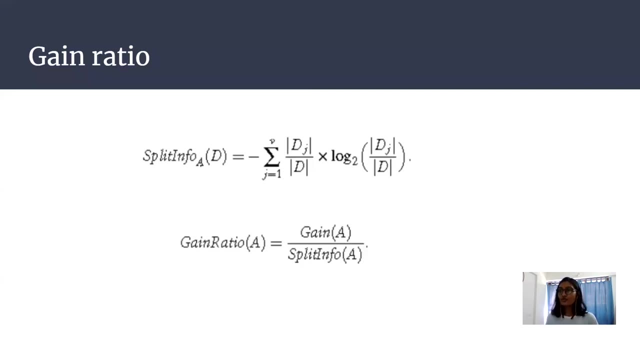 of t would be equal to zero. therefore, the information gain by partitioning of this attribute is maximum. clearly, such a partitioning is useless, and that is how we come up to our next topic, which is gain ratio, which is also known as c4.5 decision tree. so it applies a kind of normalization to information. 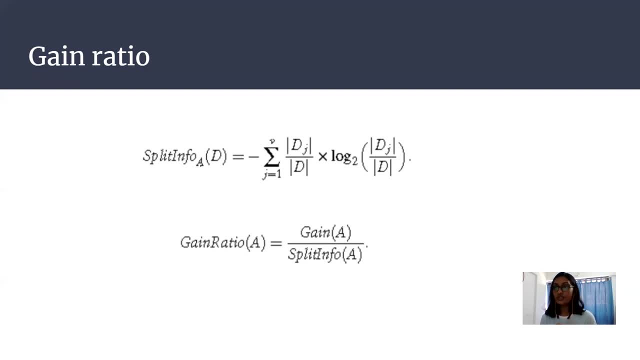 gain using a split information value defined analogously as info of t. so the computation of gain that used to be the gain value of the information, gain value of the information gain value of the 찍ult of k. this is what we have chosen for evaluation. respect the output. 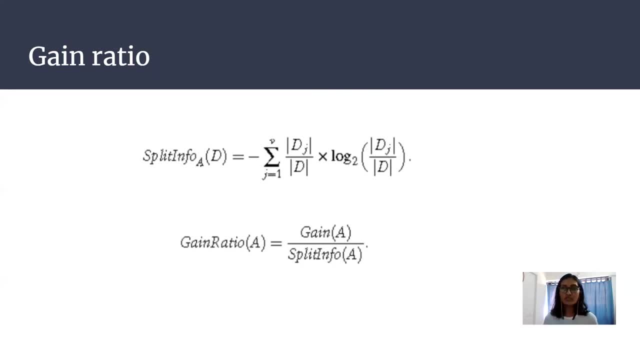 which we will just keep it data extreme if we really want to do, we will just keep it as you see the numerate over here. the additional thing that you have to calculate over here is split info. so split info has been calculated as the weighted aboriginal long of the same weighted. 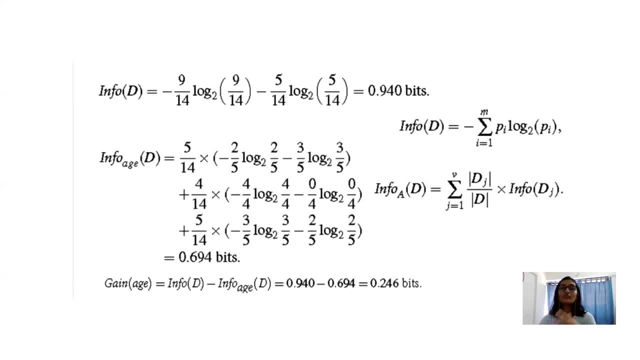 average. thereafter we are dividing it, thus we are normalizing it, and the attribute with maximum gain over here is selected as the splitting attribute, and thereafter the same process as we had credit rating. then they compare the Gini ratio and thereafter we meet the whole tree. 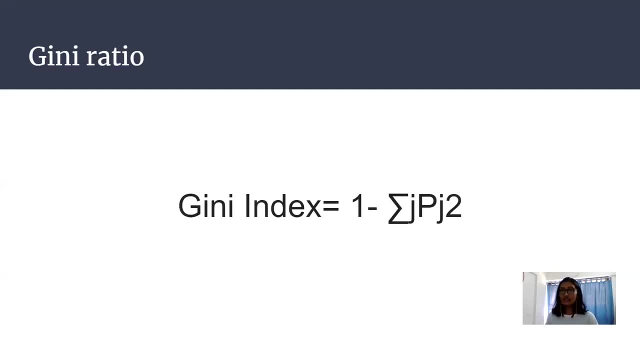 The next part that we'll be discussing is Gini ratio, which is also known as CART as classification and regression tree. So Gini ratio is also being defined as a measure of impurity or purity used while creating a decision tree, An attribute having a low Gini index. 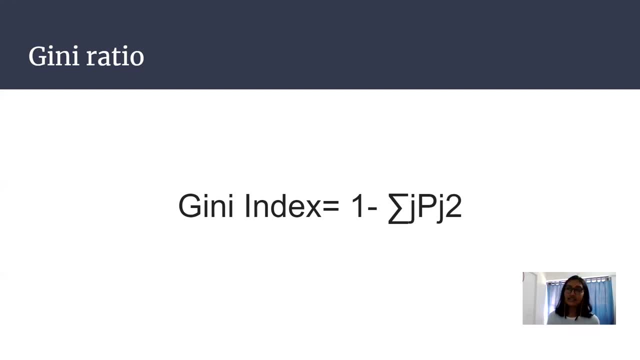 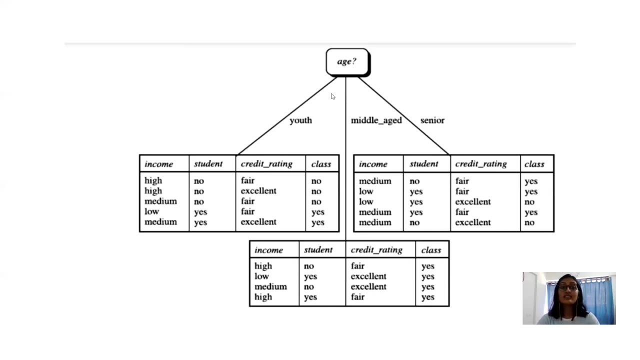 value should be preferred, in contrast to high Gini index ratio. It only creates binary splits, So there will be only and only two values that it can have, As in this example, it is not a binary split, as the split has been done in three different tables, But in 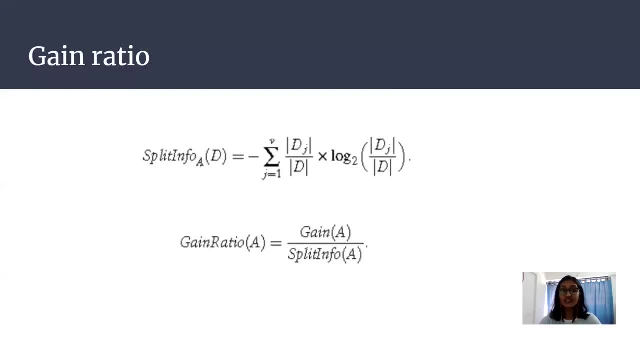 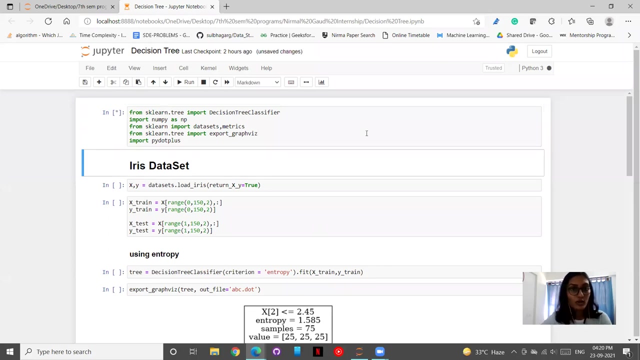 case of CART there will be only two splits, So it is strictly a binary tree. So Gini index can be calculated. Next we'll be moving forward to the code and understanding of the whole math that we have discussed. First of all we'll be importing all the necessary libraries, So the classifier, 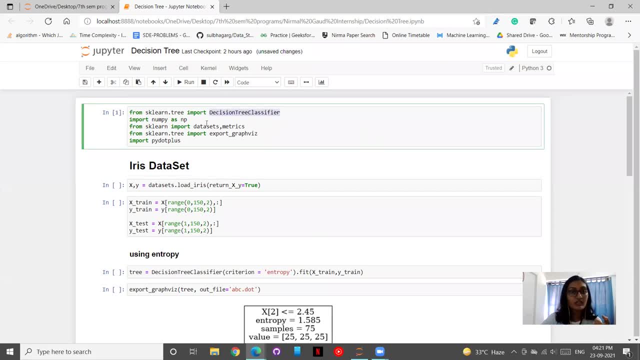 in a scale on. that we'll be using is known as decision tree classifier. We are asking for metrics so as to evaluate our model. Next, we'll be using the data set to load iris, Then export graphics, and pi dot plus is used to visualize this tree that we are making. So we are loading our data set. This 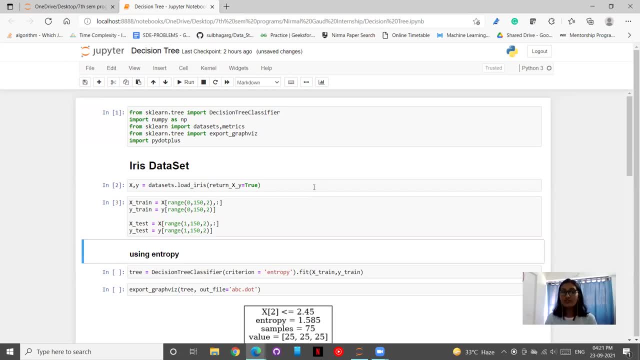 is how we are splitting it. So the usual way that I always used to split is using the train test split. But this is also one other way of splitting the data And this should also be known. The first part is using entropy. So entropy here in the criteria we are using. 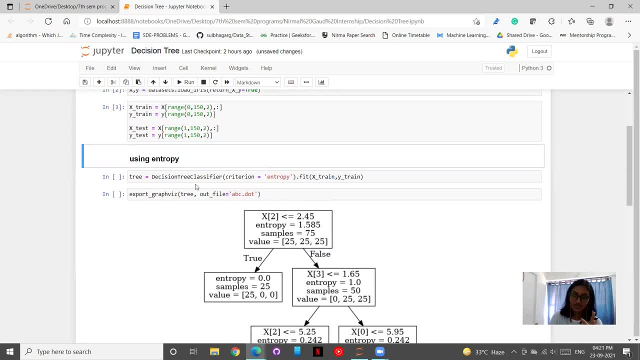 entropy. So entropy here in the criteria we are using entropy. So entropy here in the decision tree means nothing but information give that we understood the very first time, which is ID three classifier. So this is a tree that has been made And, as you can see, 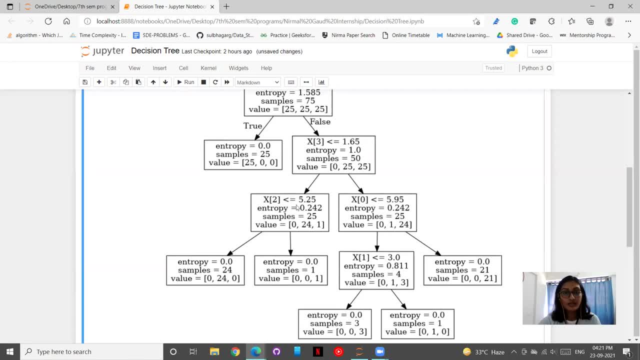 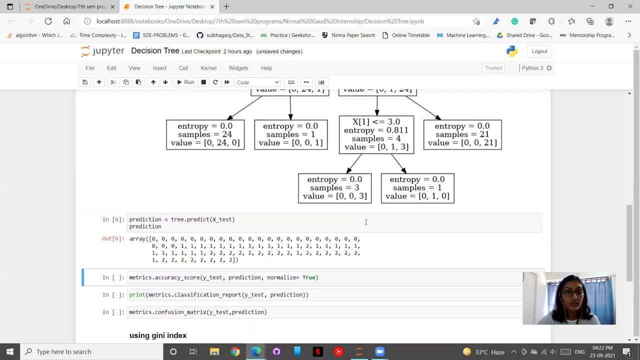 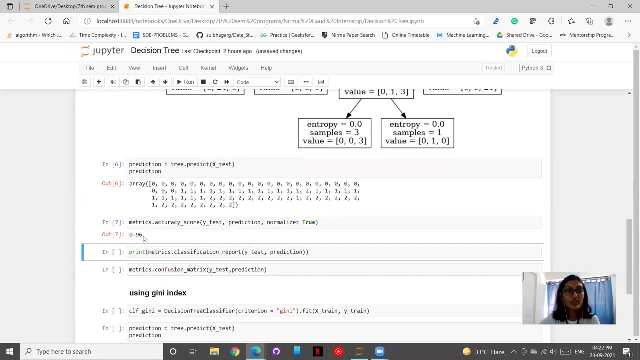 this is how the whole splitting has been done: The different entropy, sample values, etc. etc. the whole math that we did. Then, after we are predicting what our results, what the tree, our module model is, is predicting and we are finding the accuracy. So our accuracy is 96%. Now the classification. 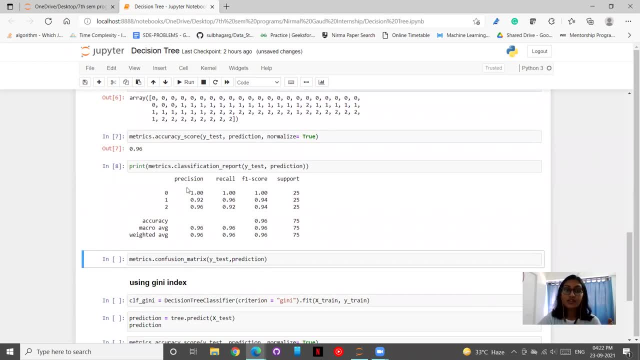 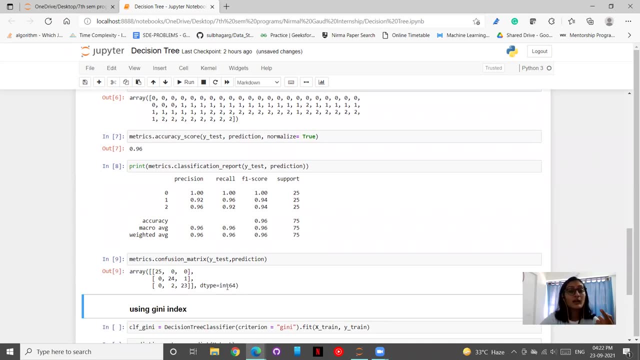 report, for if you are unknown with the terms precision, recall, F1 score and confusion metrics, which we have printed over here, please do go and watch the video which has been given in the description section, wherein have explained what all these metrics mean. So these are.